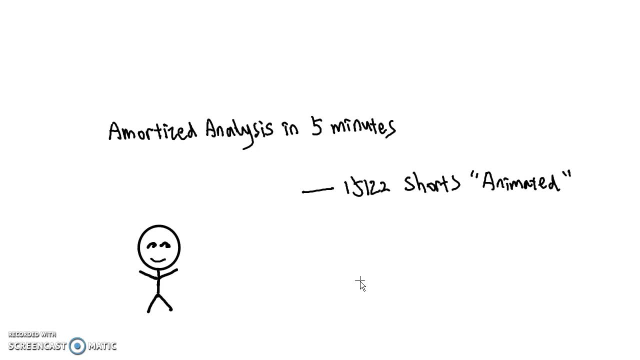 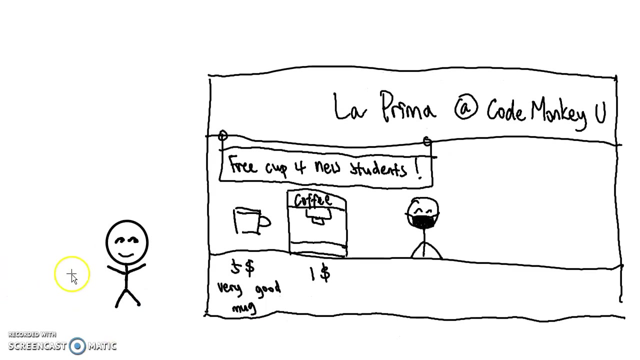 who is tired from all of his 122 homework. However, he is determined to get that A in the class, so he decides to go to his best friend, Coffee, for help. To get coffee, Eliano goes to this nice little coffee shop called La Prima, located at Wheaton Hall. Oh, I almost. 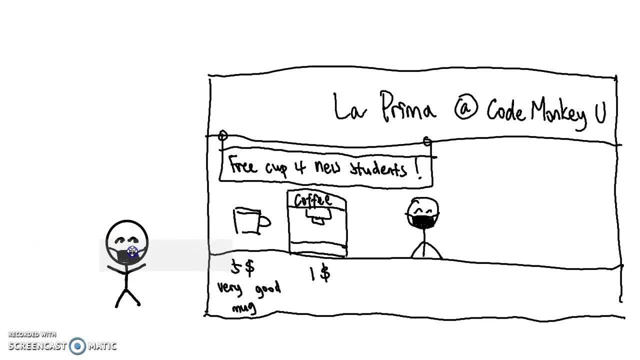 forgot something. Wear your mask, Eliano. Be safe. Alright? upon arriving at La Prima, Eliano realizes that La Prima is actually going through this new green movement where, instead of providing free plastic cups for the students, La Prima decides to sell these. very good coffee cups to the students. So he decides to go to his best friend Coffee for help To get coffee. Eliano goes to this nice little coffee shop called La Prima, located here. So he decides to go to his best friend Coffee for help To get coffee. Eliano goes. 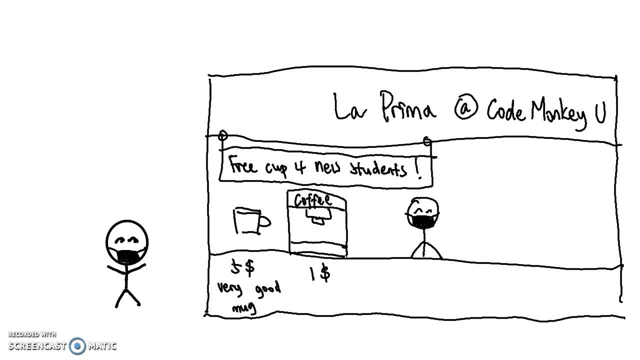 to this nice little coffee shop called La Prima located here. So he decides to sell these very good coffee cups to the students. La Prima decides to sell these very good coffee cups to the students. La Prima decides to sell these very good coffee cups to the students. 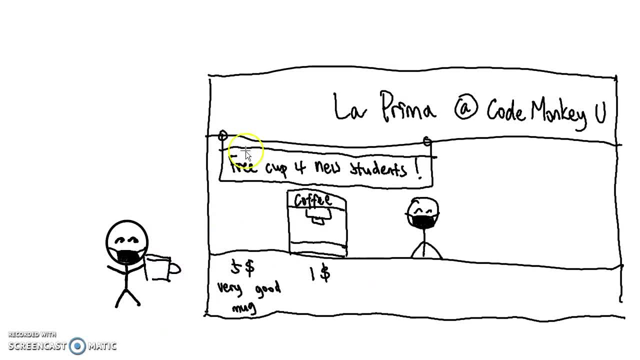 a free mug. So there's Eliano's free mug. Eliano's very happy with this deal- Free stuff, why not? So he bites his coffee and leaves. However, this actually got Eliano thinking: what is my actual cost for drinking coffee? Is it $1 for just buying the coffee, or is it $6? 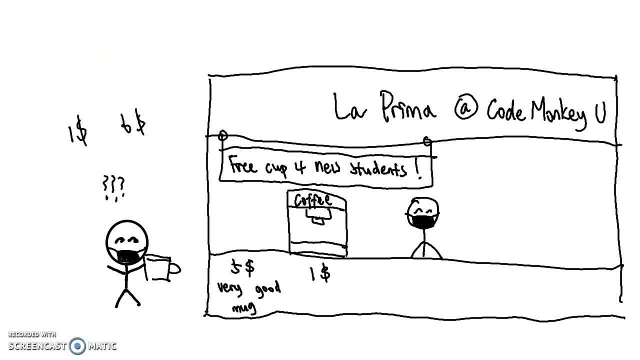 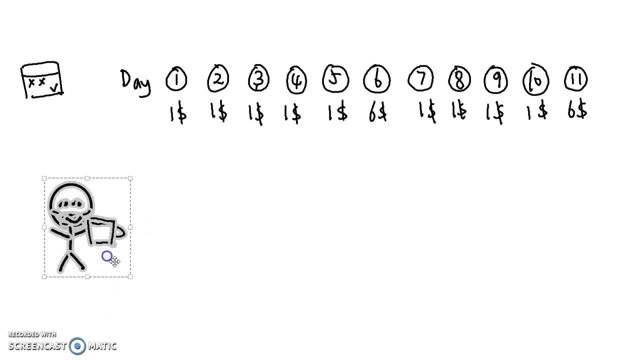 for getting both the coffee and the mug. Fortunately, Eliano's a CS student, so he decides to use what he has learned in 122 to help. Come with me, Eliano. All right. Eliano draws out this schedule, where he lists out the expected money that he's going to have to pay. 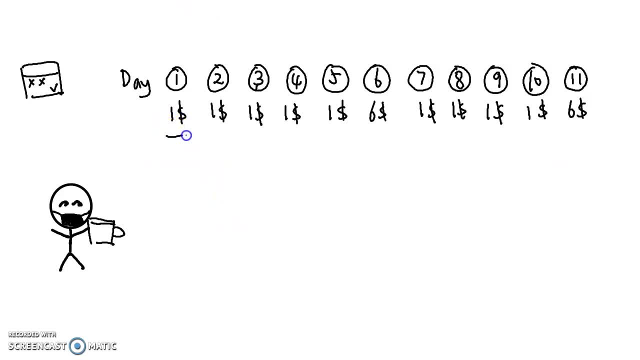 every day. On day one, Eliano pays $1, that's just getting the coffee. On day two, three, four, five, all the same. However, on day six, he realizes that his mug would have been broken by now and he needs to pay for a new mug, which costs him a total of $5 and an extra dollar. 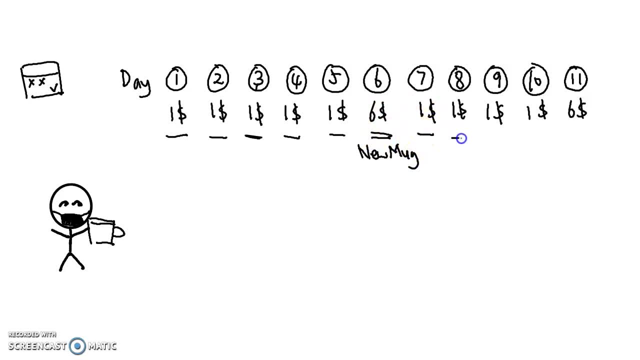 for drinking coffee. So he decides to use what he has learned in 122 to help. Come with me, Eliano, On day seven, eight, nine, ten, and it's the same thing On day 11,- another new mug. 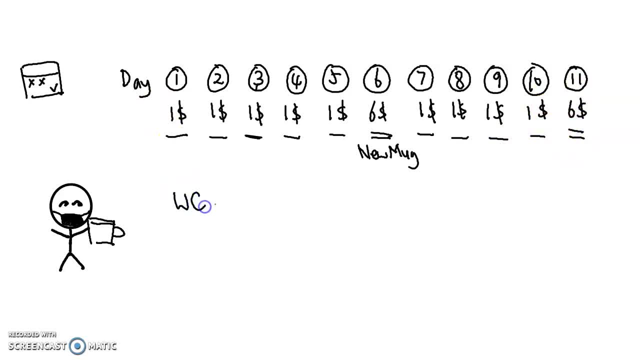 another $6.. So Eliano first tries to apply the worst-case analysis, what he has learned from 122.. The worst-case analysis tells him to look at the worst case- $6, and simply say that, oh, drinking coffee cost me $6. Hmm, this doesn't seem right. This is way too expensive. 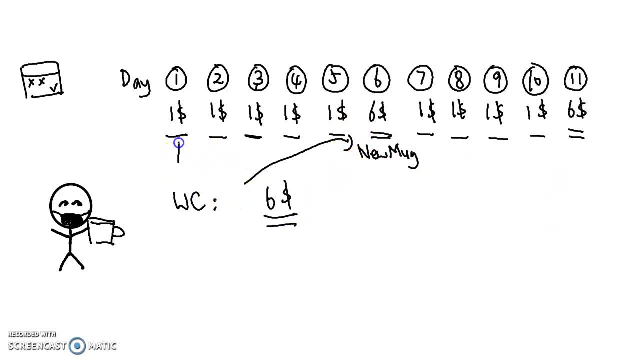 unless you drink from Starbucks. Eliano notices that most of the times he just spends $1, so he's going to be wasting a lot of money if he brings $6 to school every time. So he decides to adopt a better plan: amortized analysis. So what is amortized analysis? 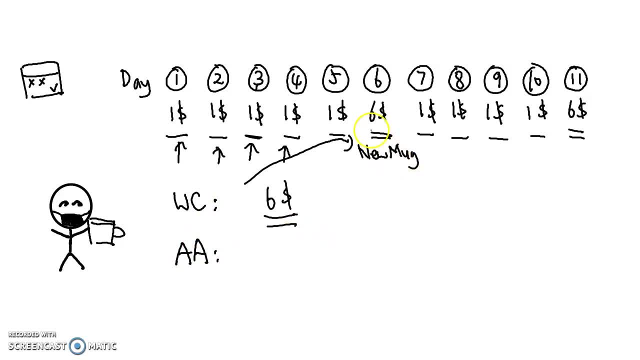 What amortized analysis basically is trying to do is to spread down the cost of this expensive day into the cheaper days. I'll demonstrate by an example. Eliano devises a plan where he only brings $2 every day and every day he spends $1. 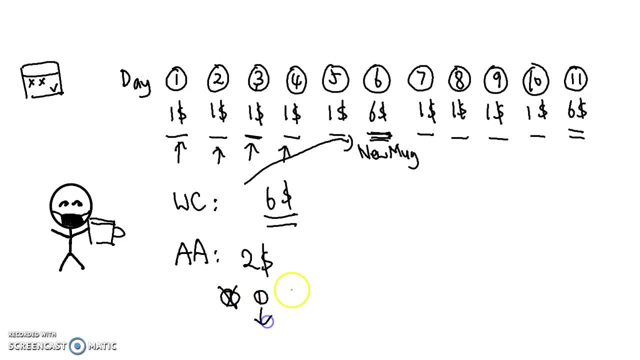 So he spends $1 on the coffee and he saves $1 in his back pocket. He does the same thing the next day. He spends $1 and saves $1. And by the time that he has gotten to day six, he would have. 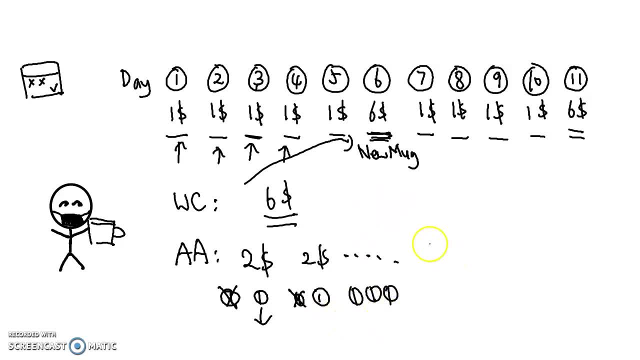 already saved $5 in his back pocket, So on day six he only needs to bring in $2.. He spends $1 for the coffee, spends the $5 in his back pocket for the mug and saves another dollar to be used on the mug at day 11.. 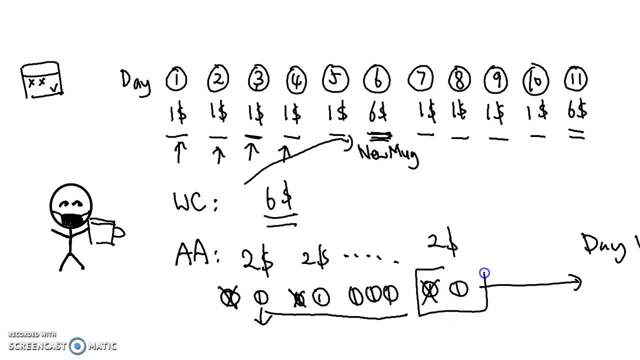 This is amortized analysis, where the cost of this expensive mug buying is actually spread down. And by using amortized analysis, Eliano knows that drinking coffee actually costs him $2 every day, which is a much more accurate estimation and, of course, better for his wallet. 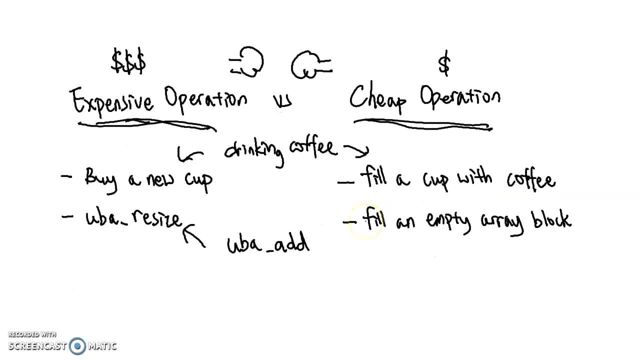 All right. so when is amortized analysis useful? Amortized analysis usually arises when an operation has both an expensive case and a cheap case For drinking coffee. the expensive case is buying a new cup and drinking coffee. That's $6 in total. The cheap case is filling a cup with coffee. 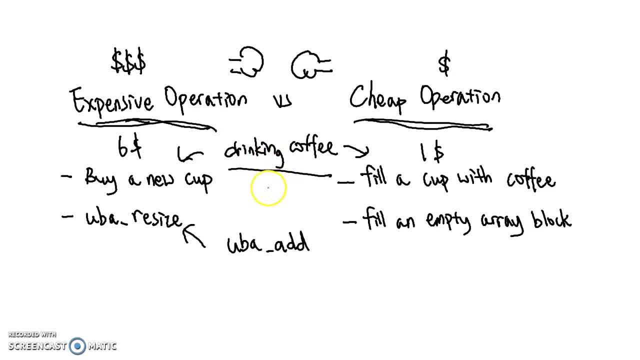 which is $1.. And amortized analysis tells us that the total average cost is going to be $2 every time I drink coffee For computer science. some algorithms, like UBAd, also has a cheap case where I fill in the empty array block. That's O of 1.. An expensive case when the array is full.